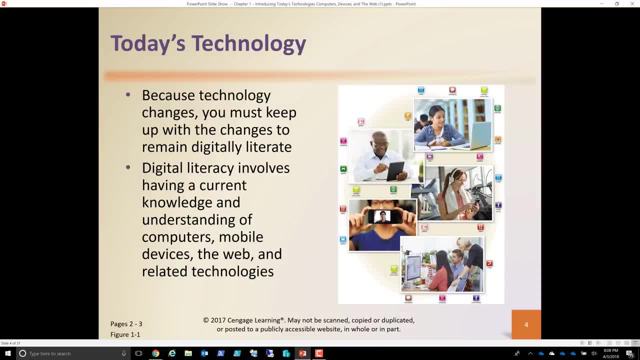 So if there's something that I've said that you don't quite understand, feel free to go over to SAM, watch their videos and I'll see you in the next video. So if there's something that I've said that you don't quite understand, feel free to go over to SAM, watch their videos and I'll see you in the next video. 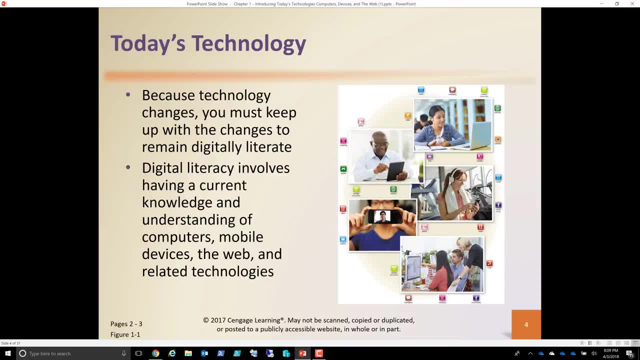 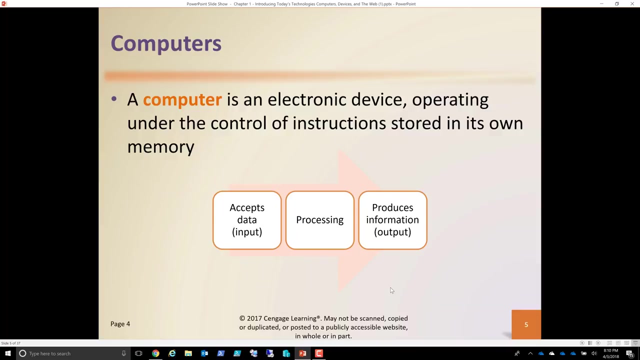 So if there's something that I've said that you don't quite understand, feel free to go over to SAM, watch their videos and I'll see you in the next video. So if there's something that I've said that you don't quite understand, feel free to go over to SAM, watch their videos and I'll see you in the next video. 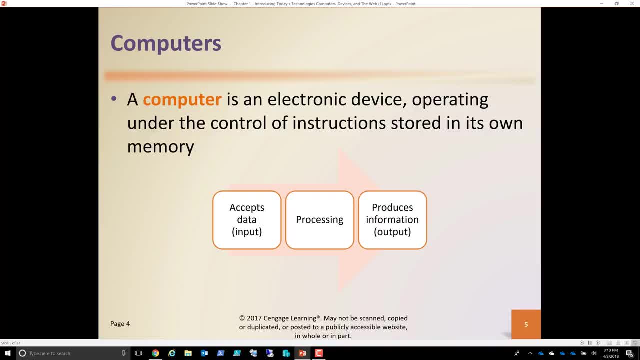 So if there's something that I've said that you don't quite understand, feel free to go over to SAM, watch their videos and I'll see you in the next video. So if there's something that I've said that you don't quite understand, feel free to go over to SAM, watch their videos and I'll see you in the next video. 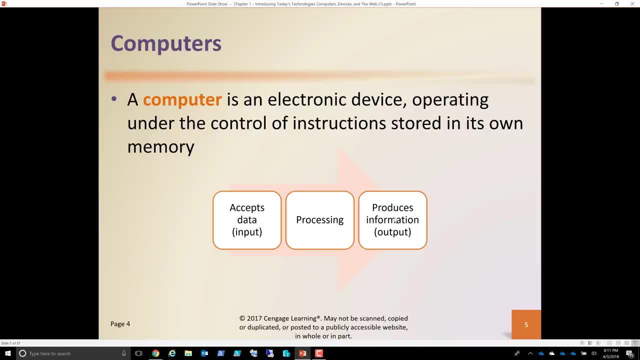 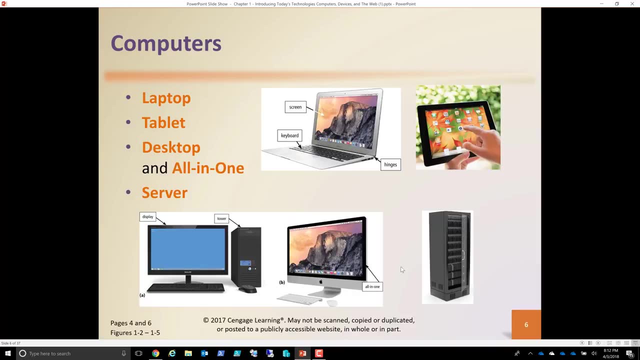 information. So data in itself is what's stored and what we ask of the computer or query or ask questions is data. So most of you have heard of the idea of a database. That's all data and we ask questions of those data and it gives us back valuable information for us to make decisions with. 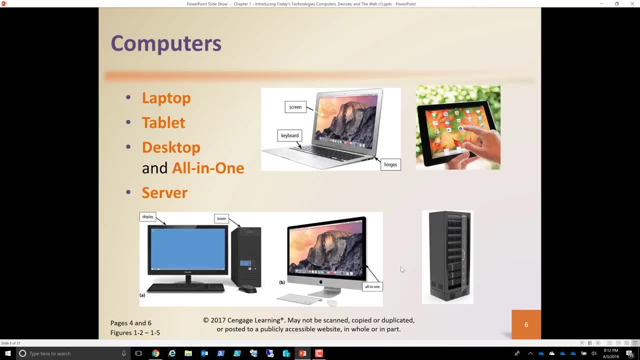 So here's some standard computers that you're probably familiar with: Laptop computers, a tablet computer. So when we talk about laptops, we can be talking about Mac OS. We can be talking about Google Chromium. today, We can be talking about Windows. 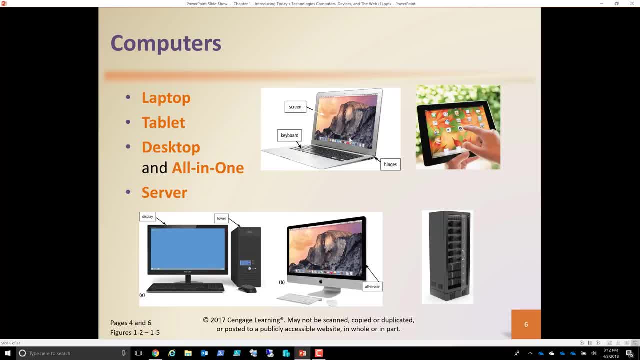 We can be talking about open source, like Unix and Linux operating systems on a laptop, computer, Tablets, of course. you're probably familiar with iPads and then Galaxy tablets for Android. So different operating systems and we'll talk about that in a little bit. 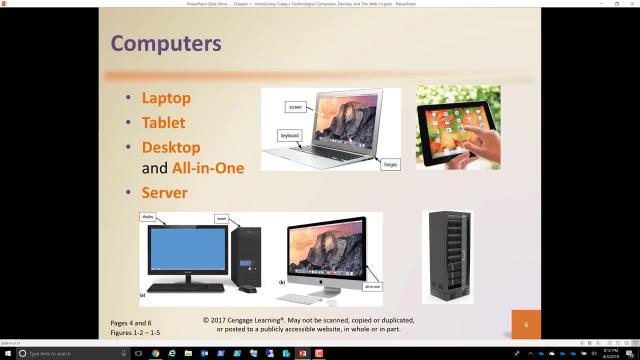 We'll talk more about those in detail later- Desktops and or all-in-ones. So this is a computer. What we have here is the traditional desktop with the tower and the monitor and the keyboard and mouse, and over here is an all-in-one. 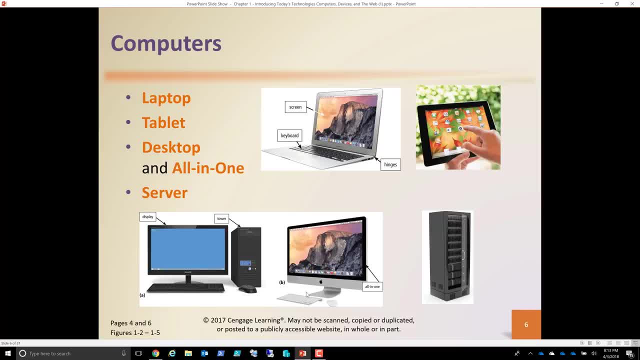 So notice we still have the monitor and we have the keyboard and the mouse, and the computer actually sits behind the monitor. It's embedded in this monitor, sits behind. It's still a computer. It's still all of the components that we need. 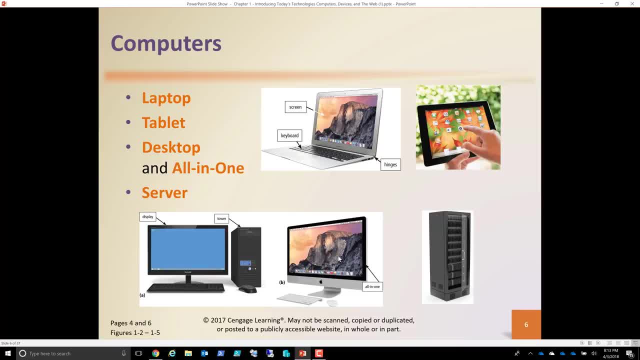 So exactly the same, just in a different form factor. Now, the one that is missing here is what's called the two-in-one, and what these are is. these are laptop computers like this, that either the screen disconnects from the keyboard and the ports on the side and 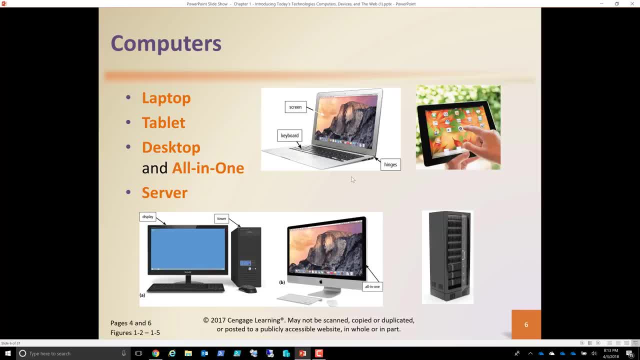 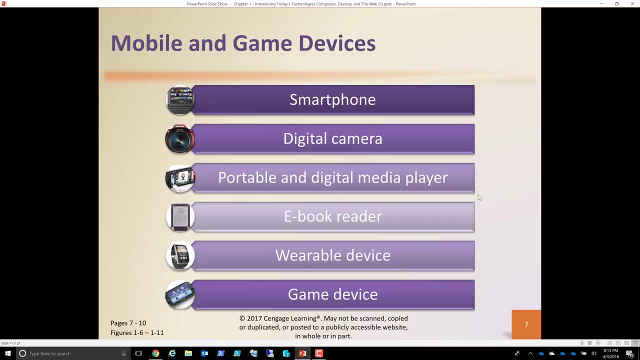 or can be flipped around and turned around and used as a tablet. So that's a two-in-one computer and I have an additional video that you'll find in this chapter that details more of the those talks about different features and functionalities, why you might buy one computer over another, which is going to be pretty important with an assignment you're going to do here in the near future. 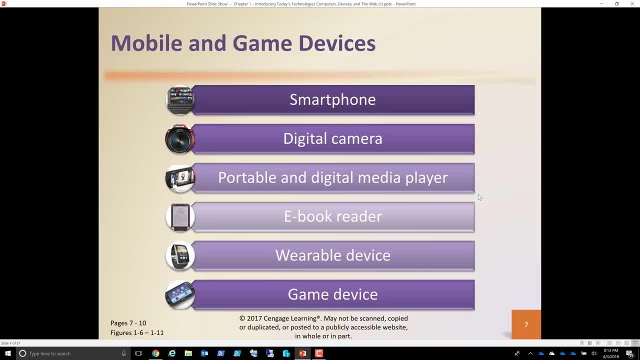 So make sure you watch that video as well. I've also got an Excel spreadsheet that details all the computers that I talk about their pricing at the time, and what you might find is the pricing continues to go down on this technology as more of it is produced. 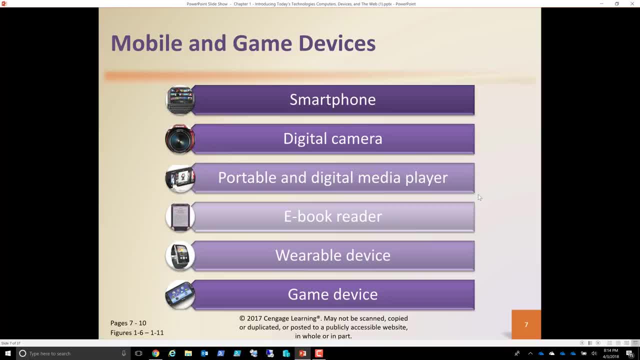 So other kinds of computing devices. So other kinds of computing devices: Smartphones, digital cameras- yes, they have a processor, they have input, they have output. portable and digital media players, ebook readers, wearable devices, whether that's your new smartwatches or 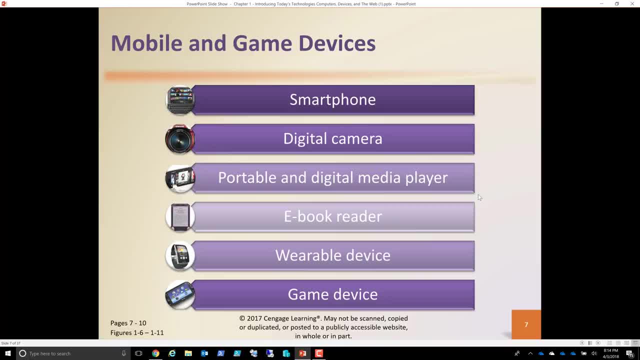 Google Glass, for example, and then, of course, gaming devices. So everything from gaming consoles, Xboxes, Sony, Playstations to the new handhelds which are making a comeback as well. So much higher quality screens and processors in those handhelds that we've had. 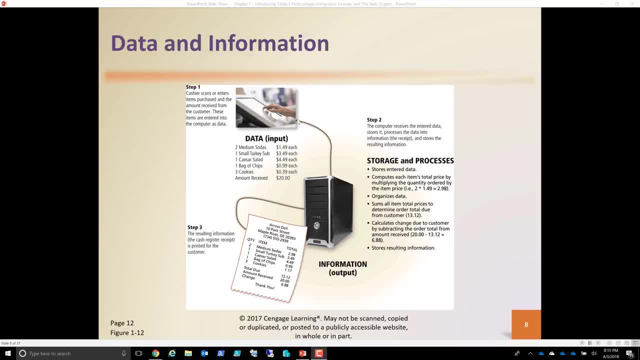 So let's take a quick look at how information as passed, stored and processed in the computer. So first we have to get information into the computer and we call that input. So in this case, in our example here are, cashier either scans or enters items using a touchscreen. 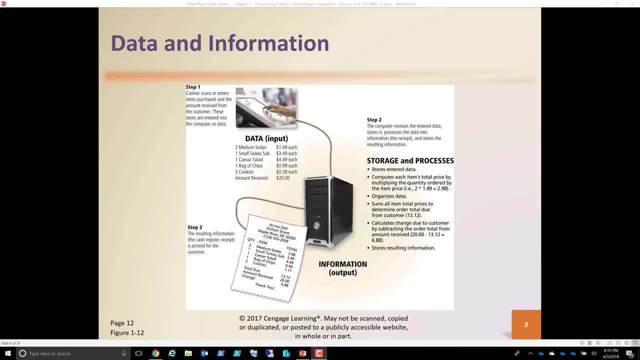 So this could be a keyboard on the touchscreen, or could be a touchscreen that has been programmed with common items. simply touch it, put in the quantity. you've seen this if you've ever checked out through the self checkout of a grocery store. so what happens is all of 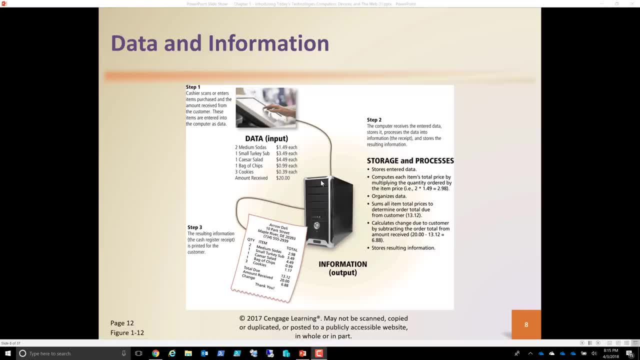 those items are stored in the computer in temporary memory. usually what it's going to do is access a database. it's going to find the current price of the items. so that's what you see here. it stores the information. it then processes the information, adding additional data to it. so we've told it, we have say one. 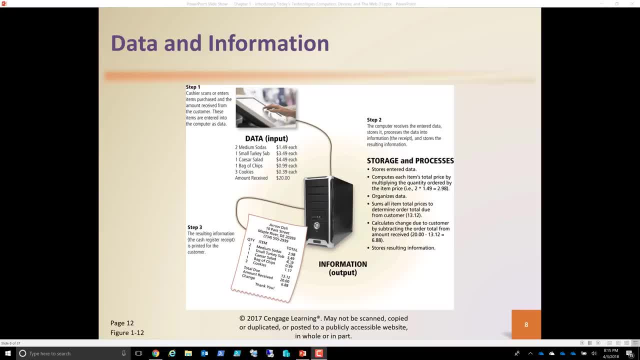 small turkey sub. that's all we've told it. it goes to the database and says: well, today, right now, one small turkey sub cost 349. what it does is it processes the data into an order, for example, and produces an output, in this case a receipt, that shows the total amount due, how much was received, the change, etc. so 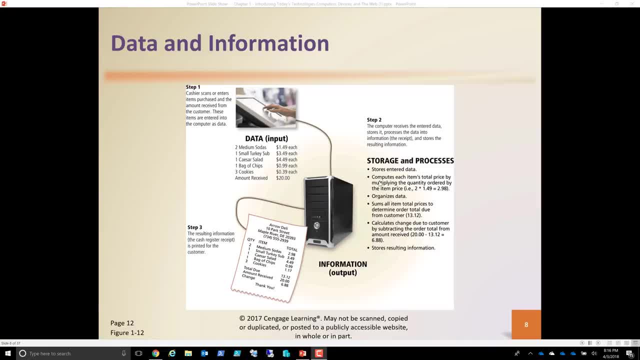 this is how things are processed in a computer. same thing when we download software from the web. we're requesting software, it's being downloaded to the computer, it gets stored on the hard drive for permanent storage and when we click on the software to open it up, the software is loaded into memory where it can be. 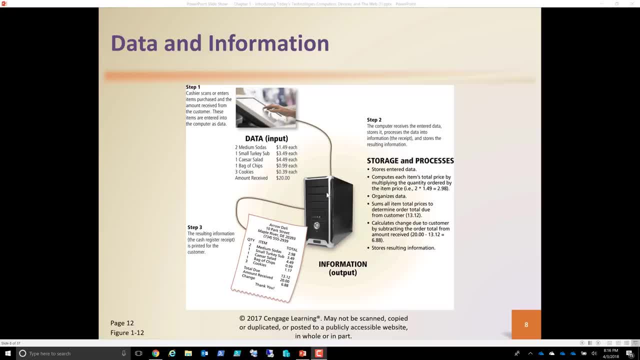 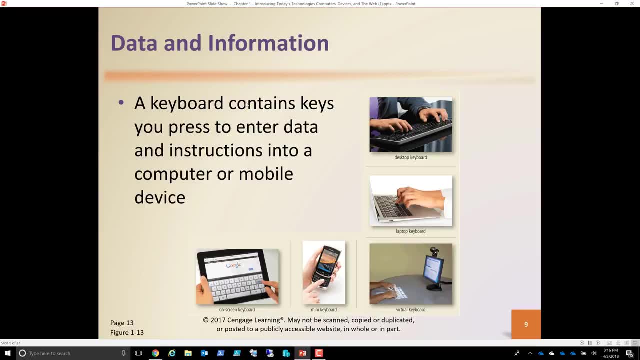 actively processed by the processor faster than reading it from the secondary storage. we'll talk about all that in more detail as well. so how do we get information into the keyboard, into the computer? well, there's a lot of ways to do it. the most common is still the keyboard, whether it's an on-screen touch. 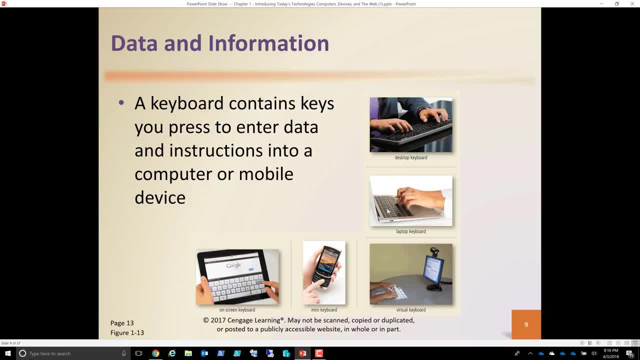 keyboard: a wired or wireless physical keyboard and embedded keyboard in a laptop and embedded or mini keyboard on a smartphone. today, what we tend to see is on-screen keyboards on the touchscreen. we don't see these slides anymore, or even virtual keyboard. so these are the idea where based on where 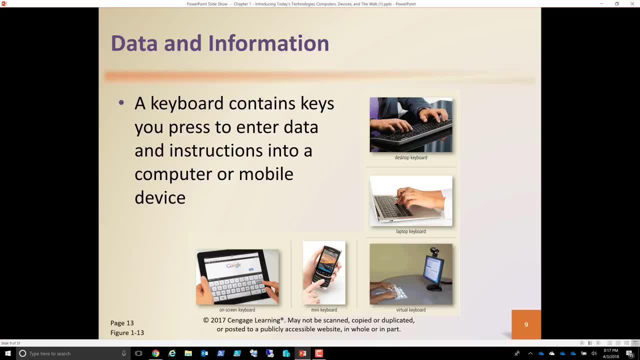 we're positioning our fingers on the tabletop, that's the key that's being pressed, and we know that most keyboards are done in what's called a qwerty keyboard fashion, because the first keys spell out q, w, e, r, t, y, so qwerty keyboard. also, other input devices that are commonly used: touch screens. 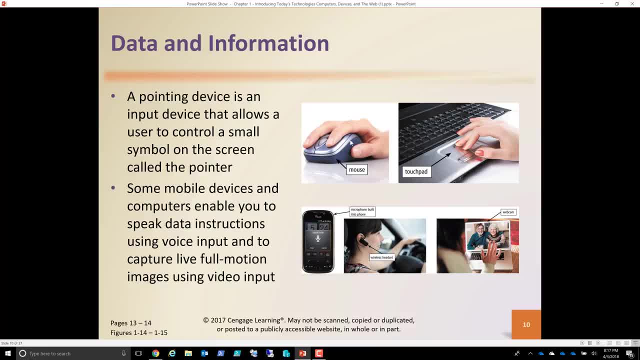 touch pads. mice are still used. so this is. this touchpad is simply another version of a mouse. so instead of moving the mouse around, we move our finger around on this touchpad, both of which use what's called an xy-axis. so if you think about math and 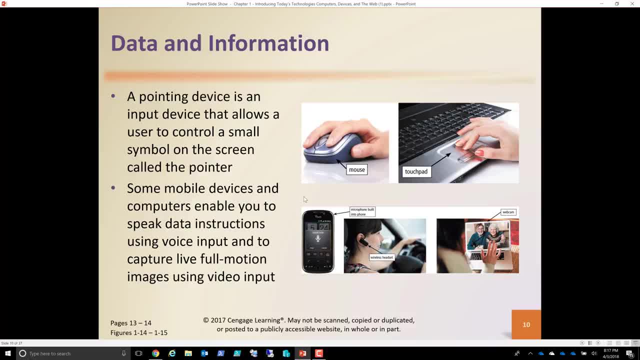 the xy-axis. that's where it knows where this cursor is on the screen. so for example, up here I'm in negative, positive, negative, negative, positive, positive, positive, positive, negative. you get the idea x, y axis, and so that's how the computer is able to know. well I'm, if I, if this was an active icon here, I could. 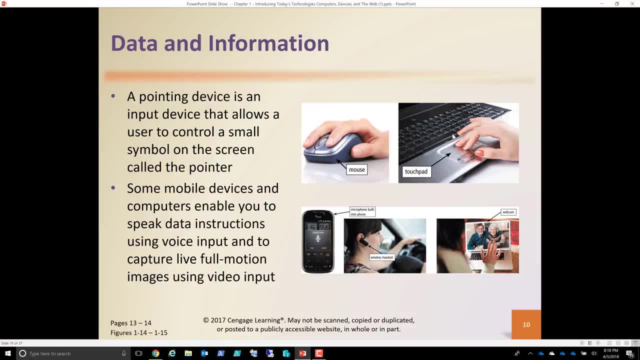 click on it and it would do something because my cursor is over that area of the screen. so that's how a graphical user interface would be programmed. some mobile devices and computers enable you to speak data instructions. pretty amazing that now we can say things like. I got to say this quietly because I got 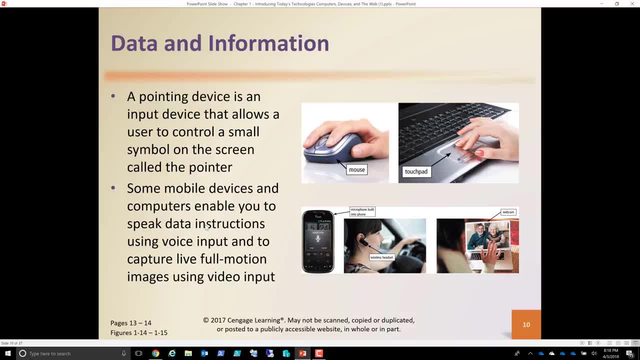 a bunch of Google devices in my house. ok Google, and boom, I'm able to turn the lights on and off in my house. I'm able to set an appointment, I'm able to ask what my next appointment is. I'm able to ask and query the web. you know who wrote what song in 1962, for example? again, that's all. 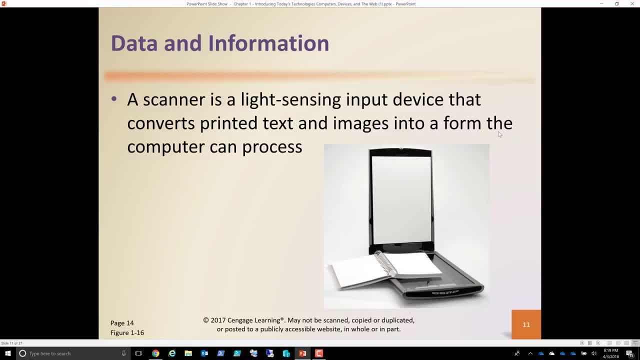 information being processed by computers who are just simply searching. the web scanner is another way to get information into a computer. we can scan pictures, we can scan books. the scanner you see here is a flatbed scanner. the reason we might still purchase a flatbed scanner today is because we get a higher. 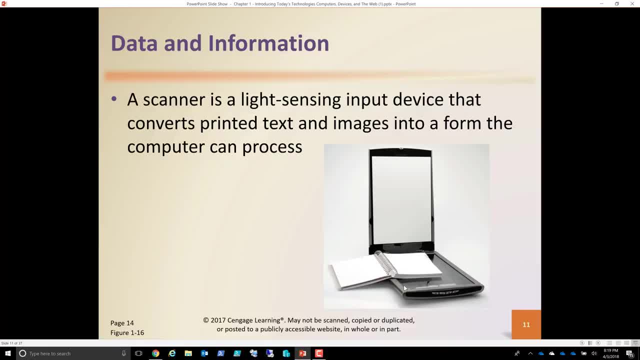 per inch ratio, so dots per inch. you might be familiar with the idea of resolution of a computer screen. for example, the screen I'm recording this on is 4k. ok, so it has a resolution with a certain number of pixels wide, certain number of pixels long. you know, in HD we talk about 1900 by 1050, for example. 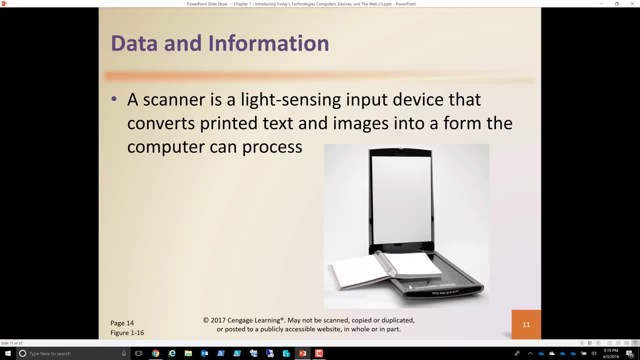 those kind of numbers, and here, the higher dots per inch, the better quality scan. so if we equate that to a monitor, when we talk 4k, we're talking about 4,000 pixels in one inch of a monitor. ok, so that's what 4k is. give you a quick example of that. 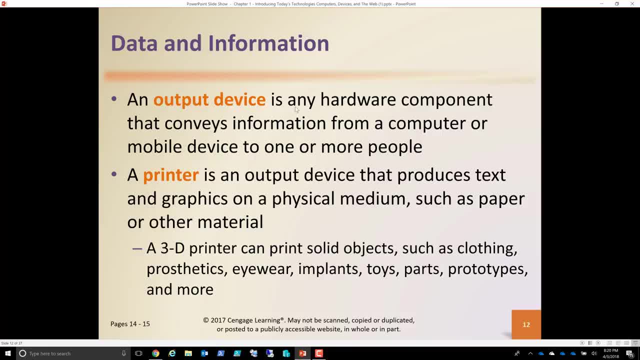 alright, so let's go ahead and we'll look at an output device. output devices: any hardware component that conveys information from a computer. standard output device today is going to be a computer monitor. now this is going to quickly change because things like Google Home and Google Assistant, where we can ask a question and Google Assistant will give. 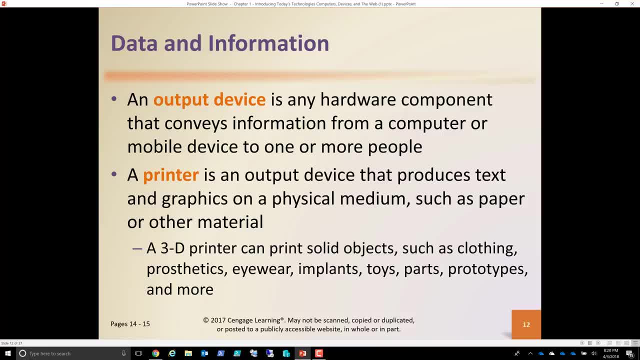 us back the answer in the form of audio output, so we no longer need to read the screen. the screen, the screen- we no longer need to read the screen- will actually get to hear the information that we've asked. so it's going to be amazing to see that artificial intelligence and that massive speed of. 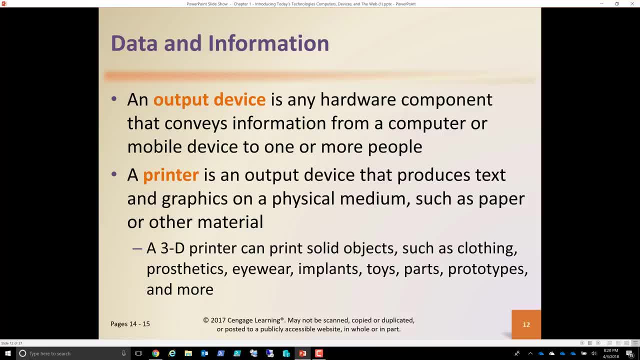 searching the entire internet and how it. Google Home is certain to make its way into business as well. a printer is another standard example today. of course, we don't just talk about 2d printers, where we have paper and an inkjet and the ink jets onto the paper, creating characters that we can then read. that's.